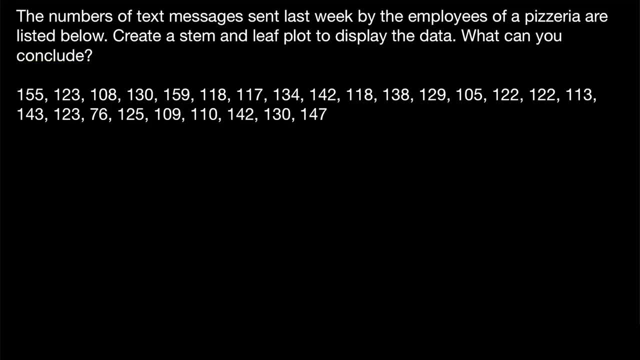 about what we can conclude from the plot. After that, we'll quickly look at a couple other examples showing us other ways that we can make a stem and leaf plot. When I say that the stem and leaf plot is a novel way of displaying data, I don't just mean that it's kind of a weird way of 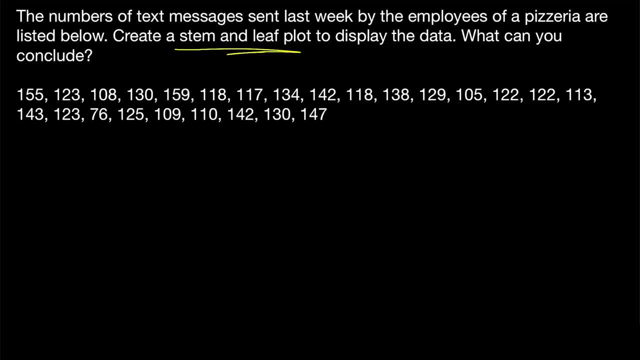 displaying data, although it definitely has some advantages, but it really is novel. This is a pretty new method. It came about in the late 1900s as John Turkey was developing what's called exploratory data analysis, So this is a method that we can use to make a stem and leaf plot. 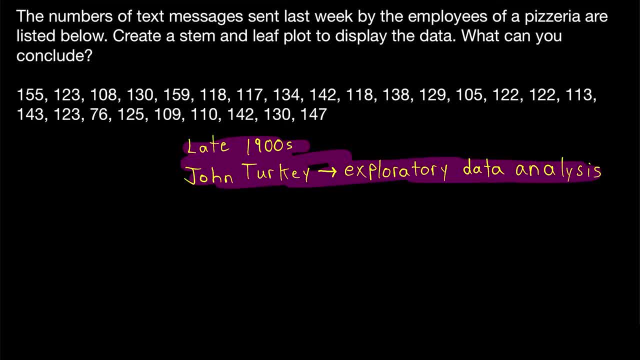 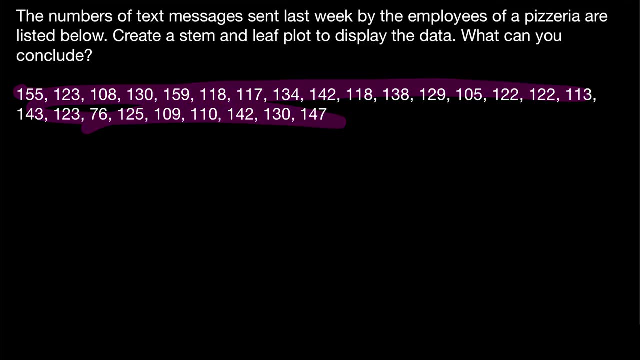 This is some modern statistics technology we're working with today. Let's go ahead and get into the example We're given the numbers of text messages sent last week by the employees of a pizzeria. Here is the list and we want to represent the data with a stem and leaf plot. 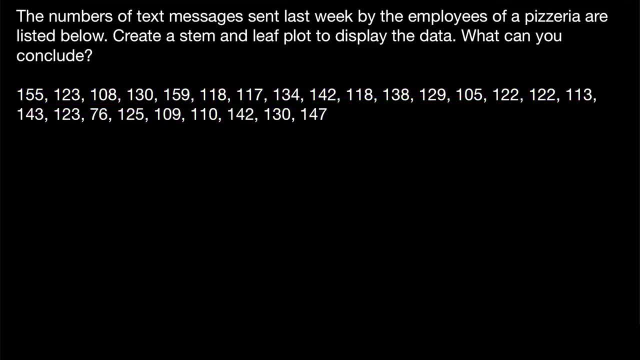 Perhaps you're already familiar with histograms. Stem and leaf plots are pretty similar to histograms. Just like in a histogram, a stem and leaf plot will sort our data points into various boxes based on their size. Those boxes in a stem and leaf plot are: 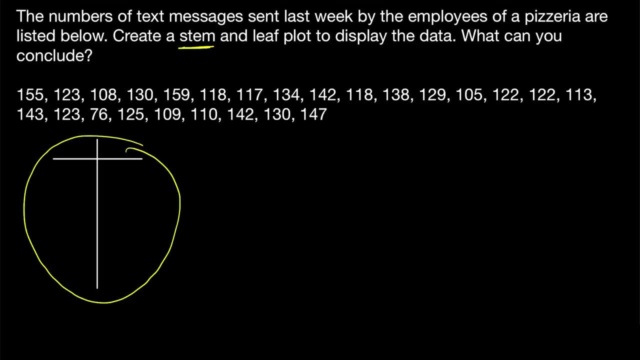 called the stems. A stem and leaf plot is a two-column chart. The left column has our stems and the right column has what are called the leaves. To start filling in the plot, we should identify the minimum and maximum data point in our set. It looks to me like the minimum. 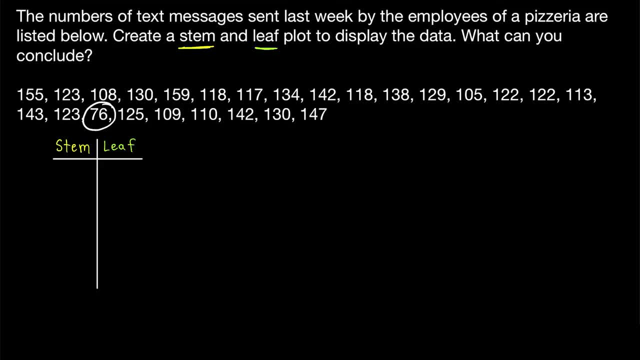 data point is 76, and the maximum is 159.. So we'll have to have stems that cover numbers from 76 all the way up to 159, and you'll see precisely what that means in just a minute. Let's just start. 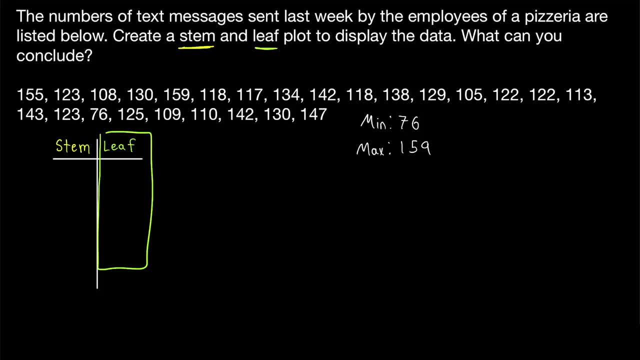 with the leaf column. Most commonly, each data point in a stem and leaf plot will be represented in the leaf column by its last column. In every stem and leaf plot, each data point is represented in the leaf column by one digit, but most commonly that one digit is the last digit. So that's what we're going to try for this. 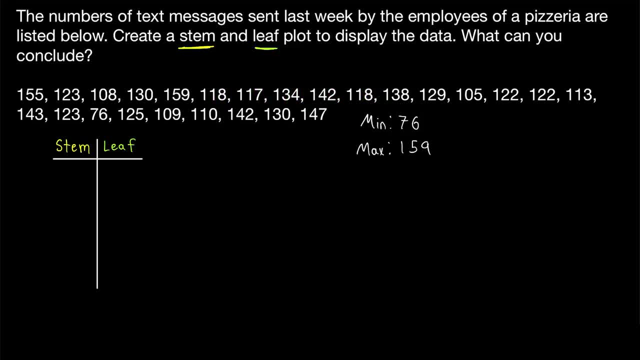 first basic plot, Starting with our minimum of 76, its last digit is 6.. So we can pop that in the first row of the leaf column And we'll see in one of the later examples how a data point might be represented in the first row of the leaf column. 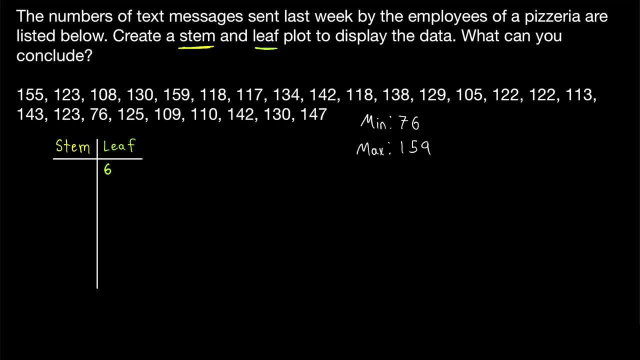 Now, if the leaf of 76 is 6,, what do you think the stem is? It's just the part of the number that comes before the 6. In this case, that's just a 7 in the tens place, and that's the stem. 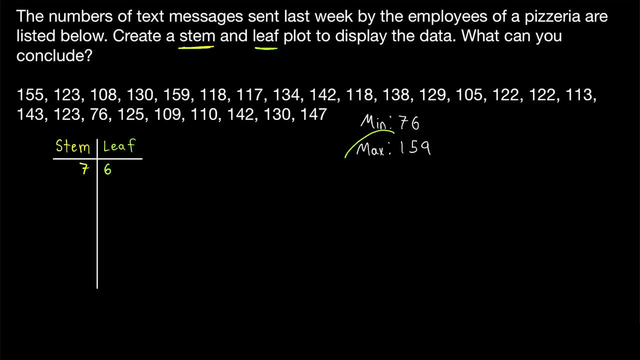 Now let's just skip all our data points and jump to the maximum for a second. What will its leaf be? Again, it's just the last digit, So we'll just pop that in the first row of the leaf column, Last digit. So the leaf is 9.. And we'll move this around to make room for other data points. 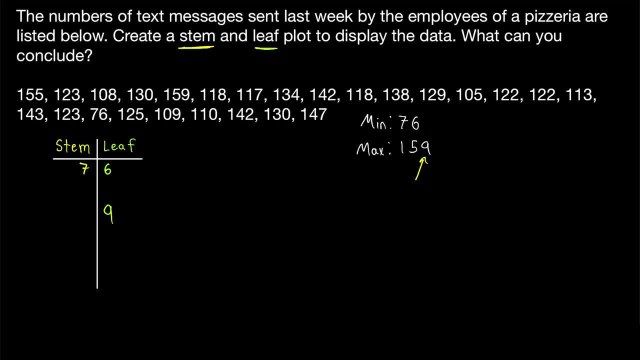 in a minute. But if the leaf is 9,, what will the stem be? Again, it's just everything preceding the 9. So in this case that's 15.. In particular, this is representing 15 tens as in 150.. So that. 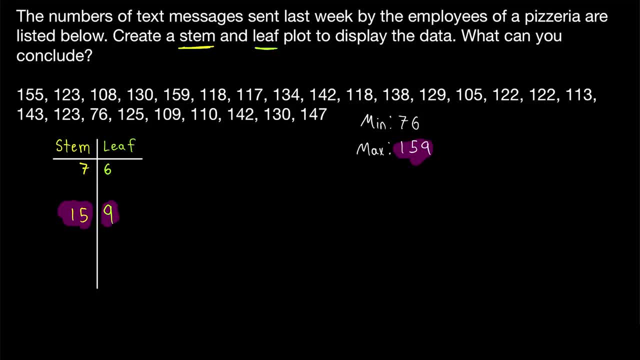 with the leaf tells us that it's 159.. Earlier, the stems are the boxes that we're sorting the data points into. So any other data point with a stem of 7 will go in the 7 row. Any other data point with a stem of 15 will go in. 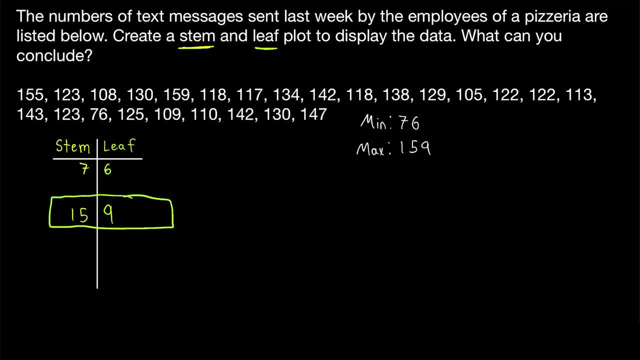 the 15 row or the 150 row, since that's what it really represents. If you look through our data, you'll see there are no more numbers in the 70 stem, But there are a couple numbers in the 150 stem, So let's put those down. I said there were a couple. It looks like it's just 1. 155.. That has. 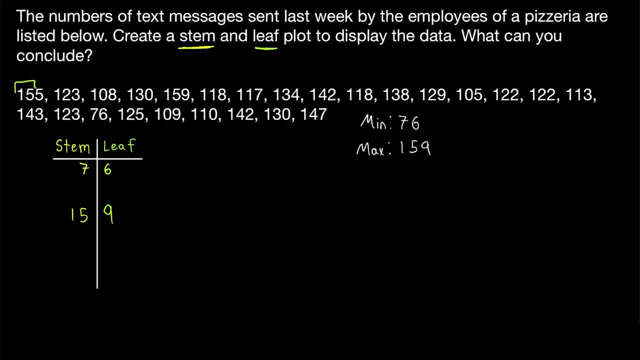 the same stem 15.. It's a 150 number And so its leaf is just that last digit, 5,, which will go in the 150 stem, And we could write that there, And that's all we do for the leaves You just. 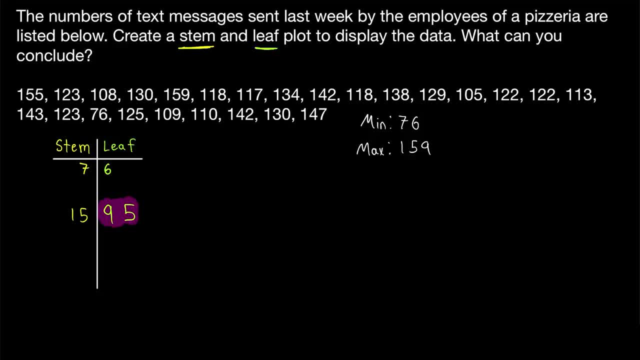 write different leaves right next to each other, No commas or anything like that. Notice that the number of leaves is just one digit. So this is 1 digit. We know it's the leaf of a single data point. This is 1 digit. We know it's the leaf of another data point. Hopefully you're starting to get the. 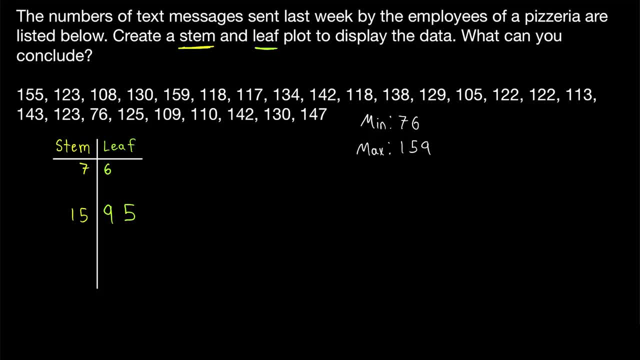 basic idea of how a stem and leaf plot works. Let's really put it together now. Firstly, our stems should always go from least to greatest, So we're going to have to make some more room here for the leaves. And notice, since we've decided to use the ones place of each data point for the leaves. 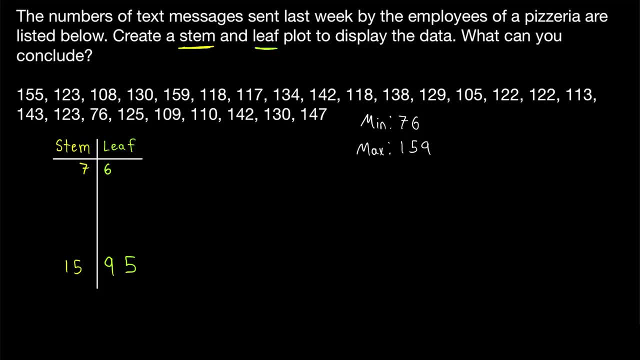 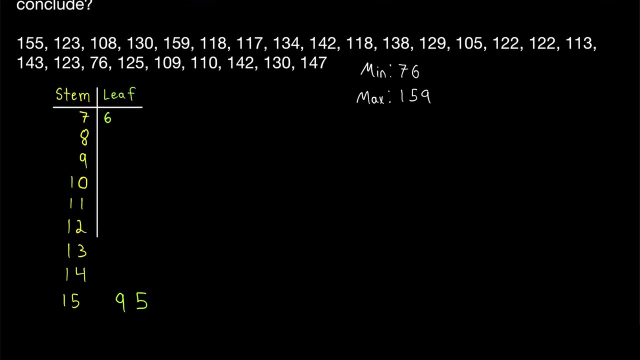 the stems represent the next highest place value: the tens. This one represents 7 tens, which are the 70s. This one represents 15 tens, which are the 150s. So we'll also need a stem for the 110s, the 112s, the 130s and the 140s. Let's scroll on down so we can see this whole thing. 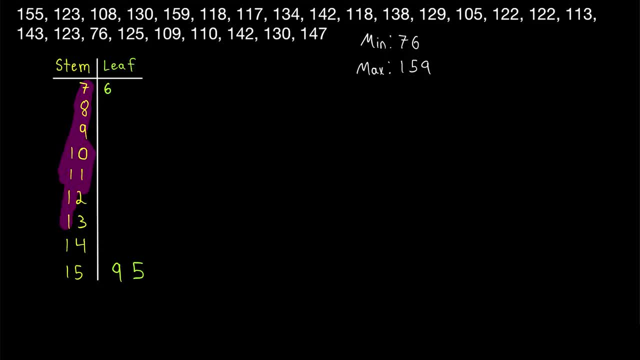 We have to include all of these stems between the minimum and the maximum, Even though, as we'll see, some of the stems might not have any leaves in them, because we might not have any 80s, for example, but we still want the 80s stem there, so we can see that we don't have any leaves in them. Okay, so let's bring in our basic stem And what we do is we're going to put a base. but even if you, we look here and look at the finder, just like other stem the upper and the middle. Brett Rompouts. 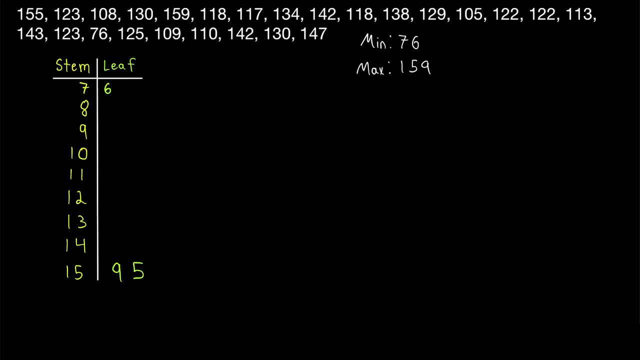 stay, endure. they're all gonna be on level so easy. This will probably washed a very, very high any of those. It will help us visualize gaps in the data. Now that we have all of our stems in place, all that remains is to fill in the plot with the leaves of our data set. We've already. 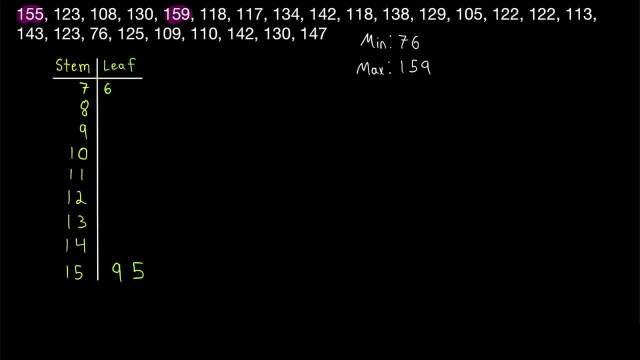 included 155,, 159, and 76.. Next we have 123.. How will we represent that and where will it go? Its last digit is a 3.. It's 123, so we'll put a leaf of 3 in the 120 stem. So there's a 3 right. 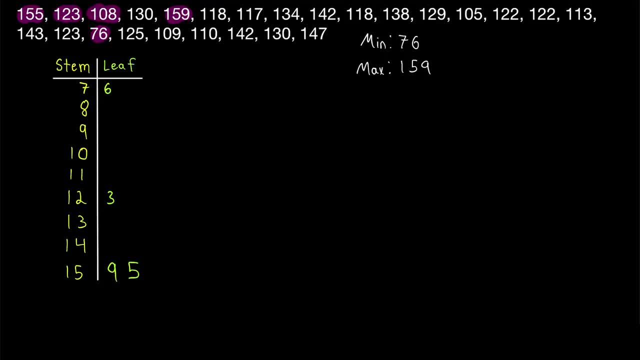 there. What about 108?? Its last digit is 8.. It's in the hundreds, so we'll put an 8 for a leaf in the hundreds stem 130.. Its last digit is 0.. It's in the 130s, so we'll put a 0 leaf in the 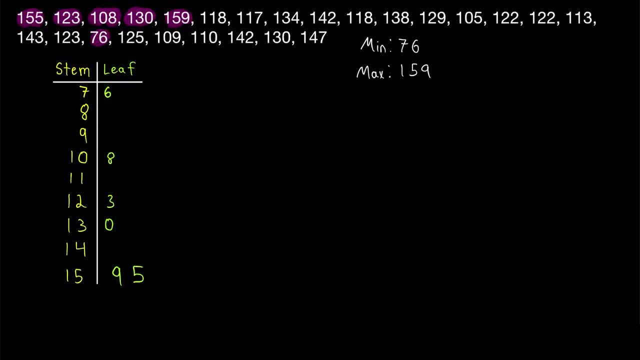 130 stem. Now let's start going a little quicker: 118.. Its last digit is 8, so we'll put a leaf of 8 in the 110 stem, 117.. That'll be a 7 in the same stem, 134.. Last digit is 4.. That will go. 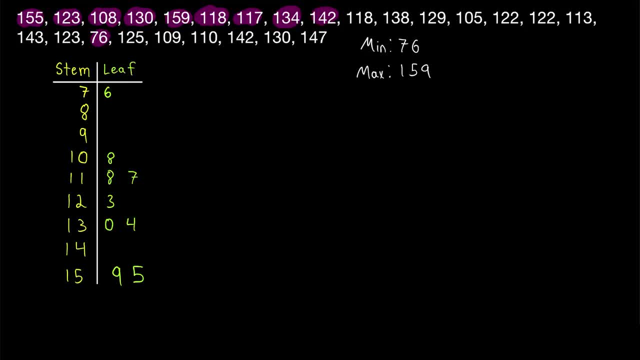 in the 130 stem 142.. Last digit is 2.. That will go in the 140 stem 118.. That's a leaf of 8 in the 130 stem 117.. That'll be a 7 in the same stem 118.. That's a leaf of 8 in the 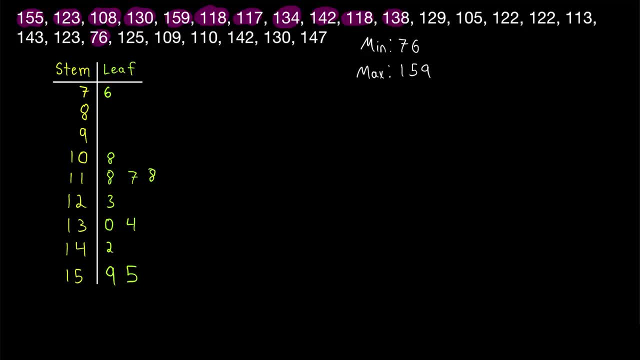 110 stem 138 is another leaf of 8 in the 130 stem 129.. That's a leaf of 9 in the 120 stem. 105 is a leaf of 5 in the 100 stem 122 is a leaf of 2 in the 120 stem 122 again. 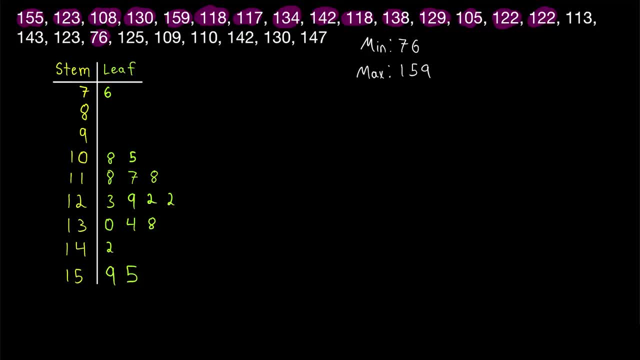 so that's another 2 in the 120 stem. Take this moment to notice that repeated data points get repeated leaves. We see that we have 118 twice and right now we've got 122 twice as well, Moving on 113.. That's a leaf of 3 in the 110 stem 143.. That's a leaf of 3 in the 140 stem. 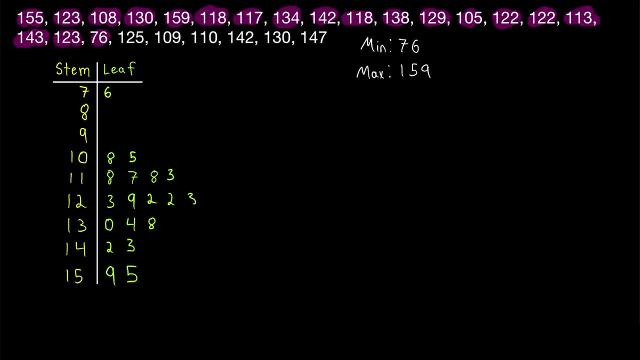 123.. Another leaf of 3 in the 120 stem, this time Then 125, because we already got 76. So 125.. That's a leaf of 5 in the 120 stem. 109.. That's a leaf of 9 in the 100 stem. 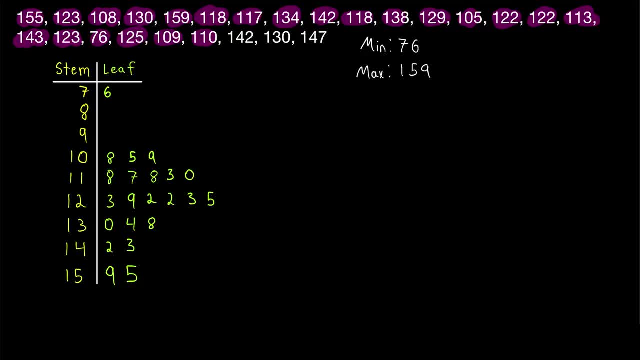 110.. That's a leaf of 0 in the 110 stem. 142 is a leaf of 2 in the 140 stem, 130 is a leaf of 0 in the 130 stem And finally, 147 is a leaf of 7 in the 140 stem. 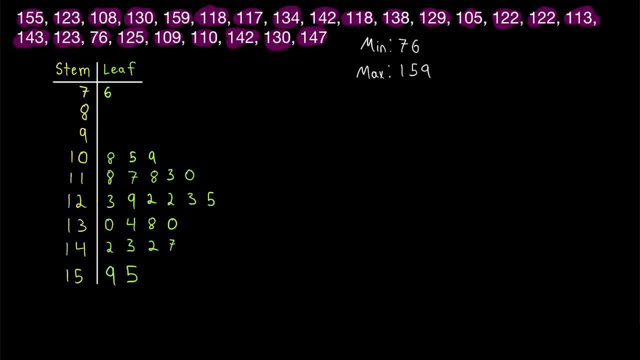 And that is our stem and leaf plot displaying this set of data. Notice the stems are ordered from least to greatest, but this would be considered an unordered stem and leaf plot because we haven't organized the leaves from least to greatest inside of each stem. It's not necessary to do that, but oftentimes you might want to. 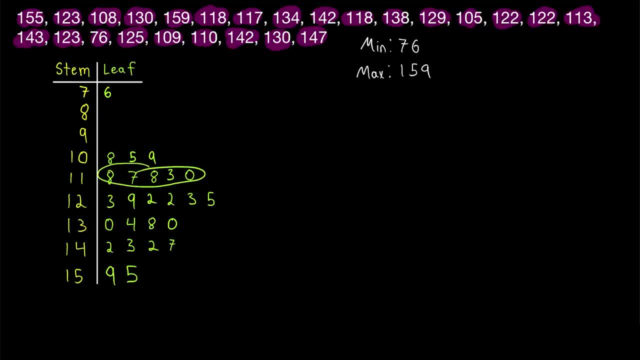 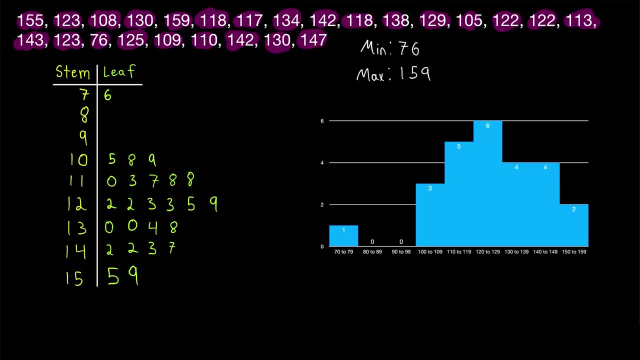 So I'm going to order all of these leaves from least to greatest inside of each stem and cut to when I'm done. All right, there is our fully ordered stem and leaf plot. Here is a histogram representing the same data set. I think you can see some of the similarities. 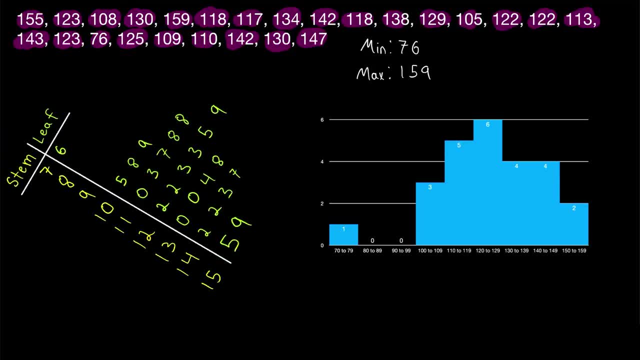 here, especially if we take our stem and leaf plot and rotate it onto its side. In a way we can see how the stem and leaf plot doubles as a sort of ugly histogram. Remember, these data points are numbers of texts sent. We can see that the most common numbers of texts sent are in the 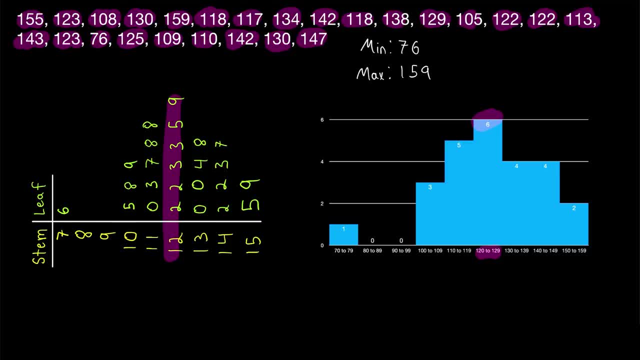 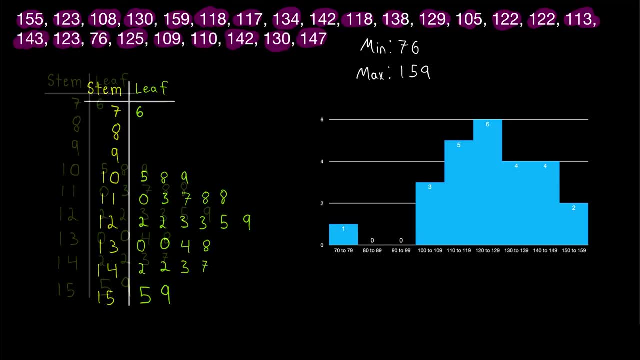 120s. The histogram could tell us that same information. But what's really cool about the stem and leaf plot is that it preserves the original data set. We still have all of our data points here. Looking at the histogram, we can see it looks like we've got an outlier between 70 and 79.. Looking at the 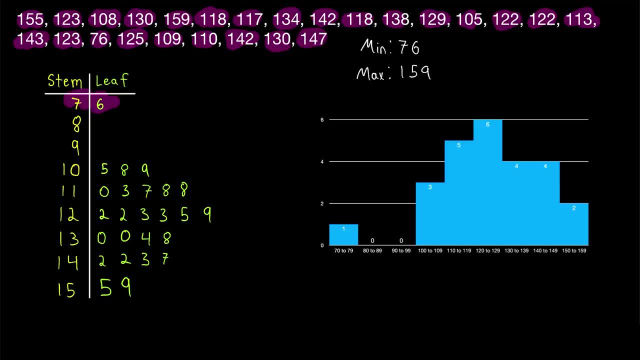 stem and leaf plot we can say 76 is an outlier. We can see the data point right there. We can also immediately identify the minimum and maximum values. We can also see the data points here. We can also see the values in the stem and leaf plot, Our minimum of 76 and our maximum of 159.. That of 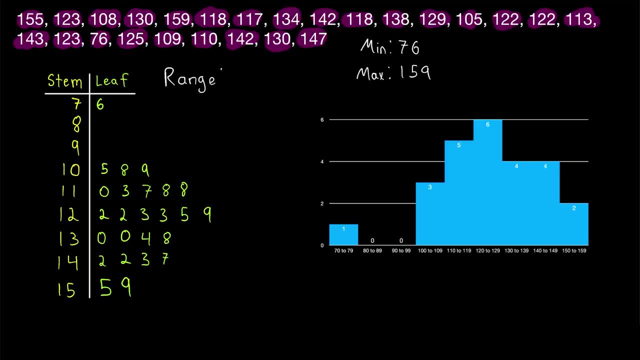 course makes it easy to see that the range of our data is 159 minus 76,, which is 83.. Another thing we can quickly learn from our stem and leaf plot is that more than half of the data lies right here. That's between 110,, the lowest possible value in this stem, and 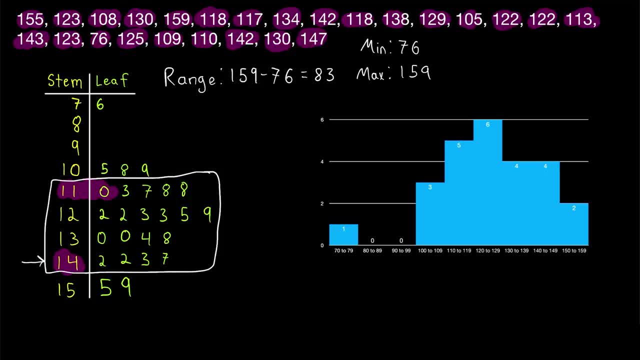 149,, the highest possible value in this stem. Note that we don't actually have a 149,, but that is the highest possible value in this stem. So we might say more than 50% of the data is between 110 and 149.. Now let's erase some of this stuff to make a bit of room. There's one important thing. 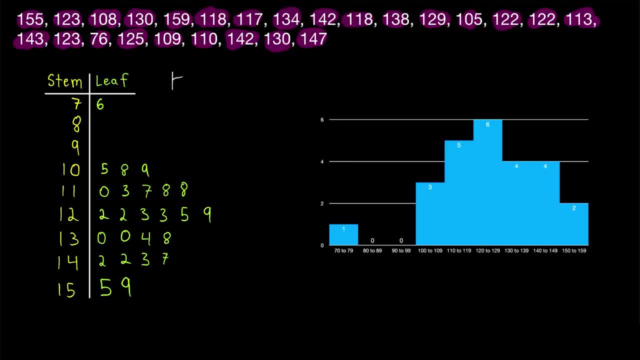 you've got to know about stem and leaf plots, That is, you should always include a key with your stem and leaf plot. I think you'd agree that these plots are a little weird, So the key helps us read it and make sure we. 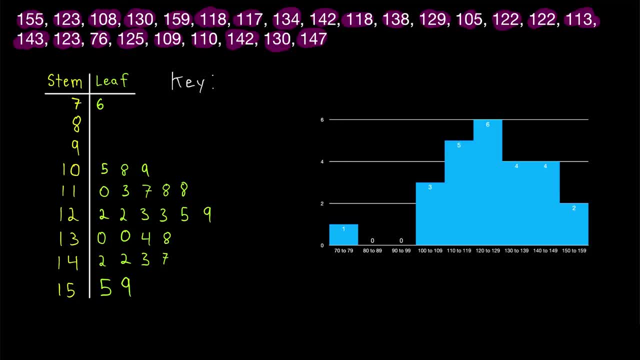 understand what it's telling us. We want the key to communicate what a combination of a stem and a particular leaf means. So for this key we might say that a stem of 10, and then put a line between it to represent that that's the stem. it's on the left side of the line And then on the right. an. 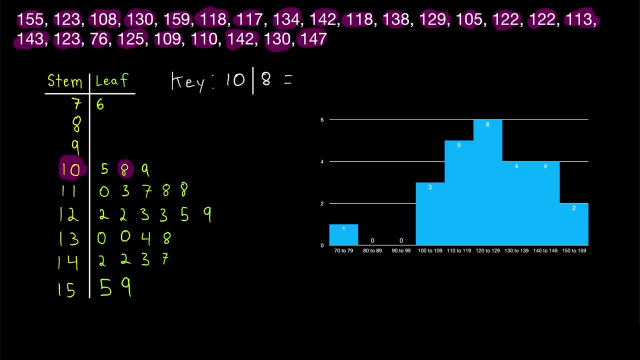 example of a leaf like eight. what does this represent? It's 108.. So now we know the leaves are representing the ones place and the stems are representing everything to the left of that. And again, this is the most common way that a stem and leaf plot. 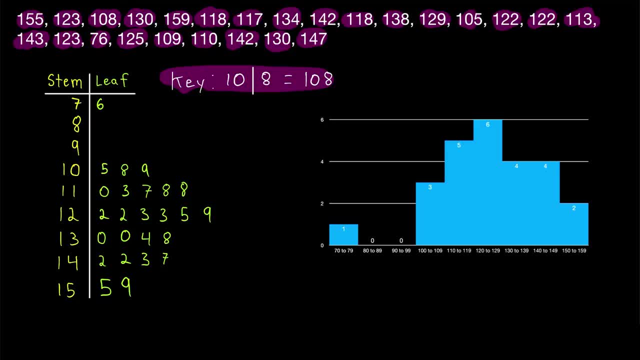 will work. So this is the most common type of key, where the leaves are the ones place and the stems are everything to the left of that. But I hope you appreciate that this is a pretty nifty way to display data. Remember how I said: the leaves should not be separated. 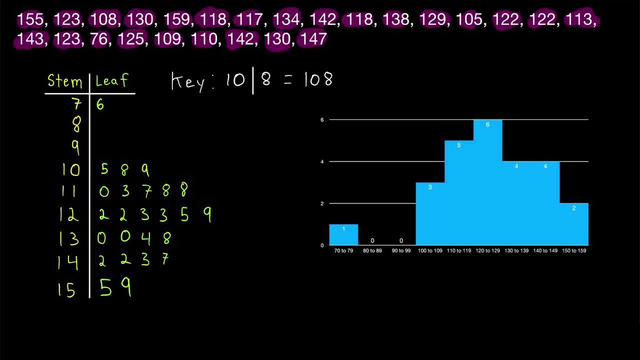 by commas or anything like that. But notice the plot is a lot more useful because I have taken care to equally space the leaves. If I hadn't equally spaced the leaves then a quick glance at the plot could be deceiving. For example, what if I made the leaves in the 120 stem really close? 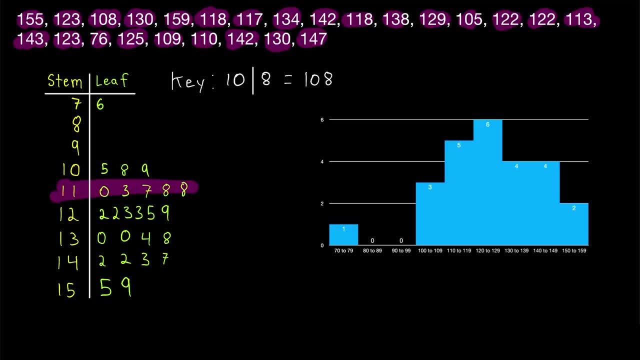 together. Well, now it looks like the 110s were the most common data points And it just looks ugly. There should be some space between your leaves and you want to try to keep that space as consistent as you can. Stem and leaf plots, although they may seem a little weird to you, were very easy for. 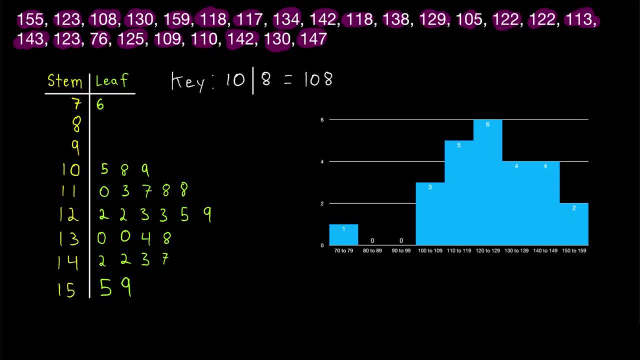 computers of the time to create, which was another reason they grew in popularity. The next two examples we look at will show us how the key of a stem and leaf plot could be different. But before we do that, I want you to consider what this plot would have looked like if we had chosen a different. 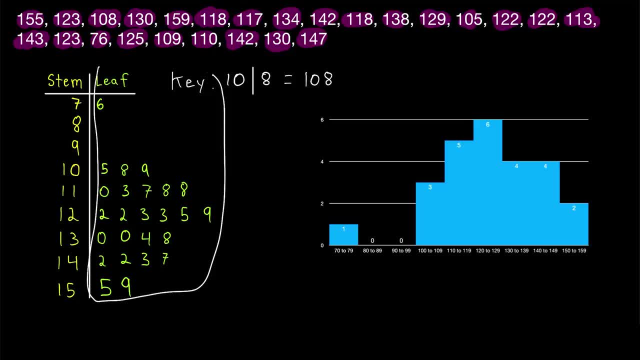 key leaves to represent the 10s place instead of the ones place. Well, our data points have ones places. So if we want the leaves to represent the 10s place, then we need to round all of our data points to the nearest 10s place. then our stems would represent everything to the left of the 10s place. 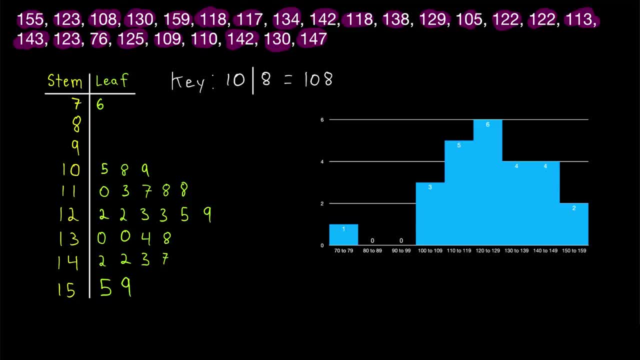 So the hundreds place, thousands place and so on. Now, in this data set, how many different hundreds place values do we have? Well, we have a bunch of numbers with a one in the hundreds place And we have one number with a zero in the hundreds place. So you should expect that stem and leaf plot to have just 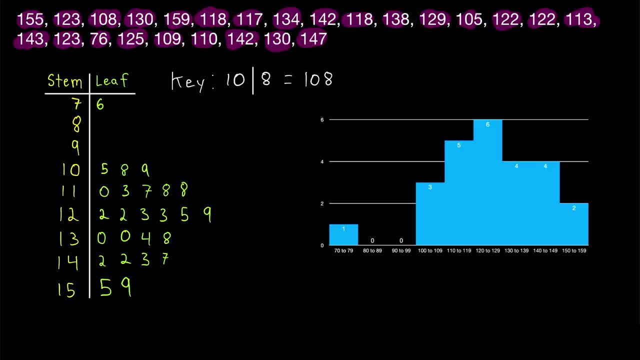 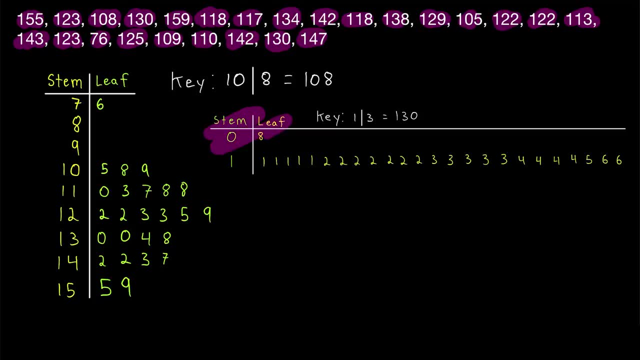 two stems And you can imagine how that would be a completely useless stem and leaf plot. And just to convince you it's useless, I made it for you. So here is the stem and leaf plot of the same data set that we just did. But here we have a bunch of numbers with a one in the hundreds place And we have one number with a zero in the hundreds place. So here we have a bunch of numbers with a one in the hundreds place And we have one. 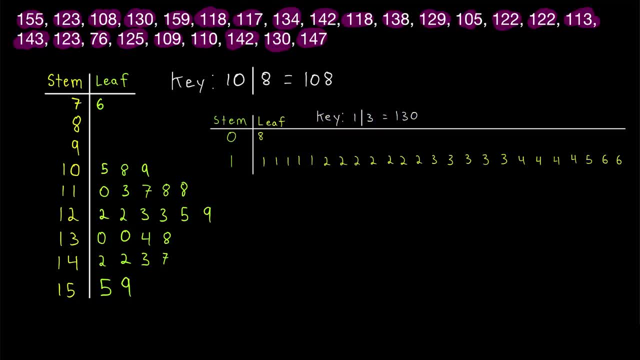 used a different key to create my stem and leaf plot. I've said that the leaves will represent the 10s place And I've rounded every data point to the nearest 10s place to accommodate that. for example, 76 rounded to the nearest 10s place is 80. So it has a leaf of eight and a stem of zero, since it has. 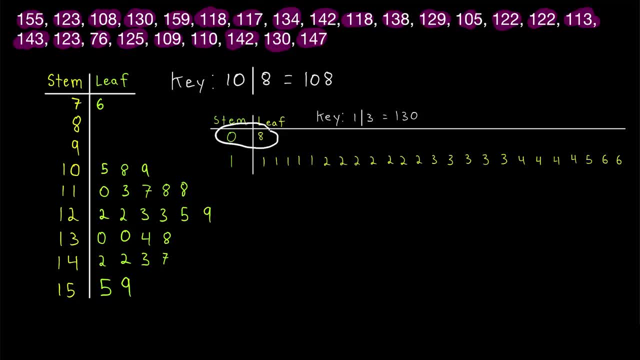 zero hundreds, But every other number starts with a one in the hundreds place, So all the other numbers are under the one stem. This type of key might be exactly what we want for a different data set, but it's clearly not the key we want for this one. 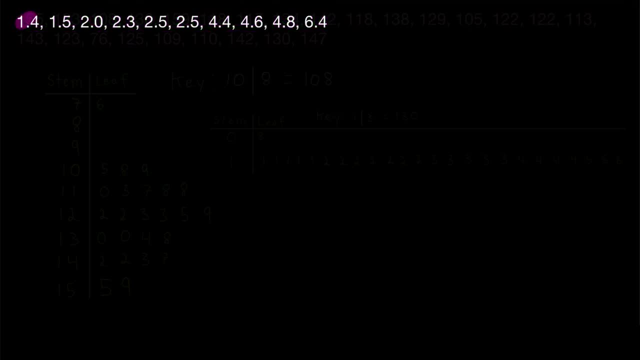 Alright, let's look at a couple other examples real quick. Here are some data points that aren't whole numbers, So take a minute and think about what a stem leaf plot for these would look like, and make it yourself if you're feeling ambitious. 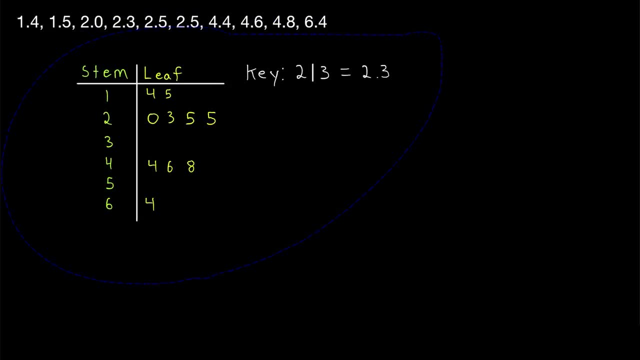 I'm about to paste it on screen now. So here we go. Here's the plot for this stem and leaf plot. The stems are the ones one's place And the leaves represent the 10th place, which is a fractional place value. 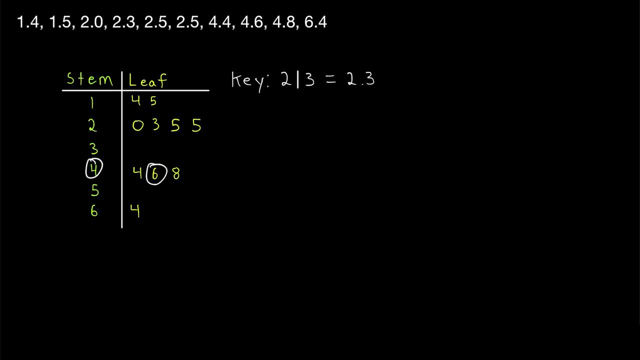 like this four and this six represent four ones and six 10th, which is 4.6.. If all of these data points happened to have a hundredth place as well, then we probably would have wanted to use the same key, And so we would have had to round them to the nearest 10th. 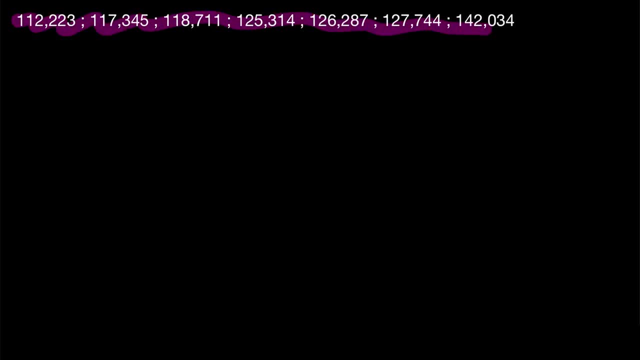 Now let's see one more example. Here is a another small data set. Notice, I've separated the data points with semi colons because the numbers are big enough that they have commas in them. Try to make a stem and leaf plot for this data set. Or just think about what. 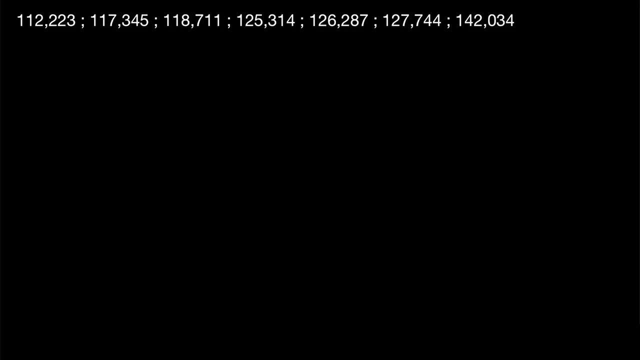 the key would be: What would the stems and leaves represent? Pasting the answer on screen in three, two, one. If we use the most common type of key for this data set, then we would have one leaf. That is, putting the ones place as the leaf and everything else as a stem. 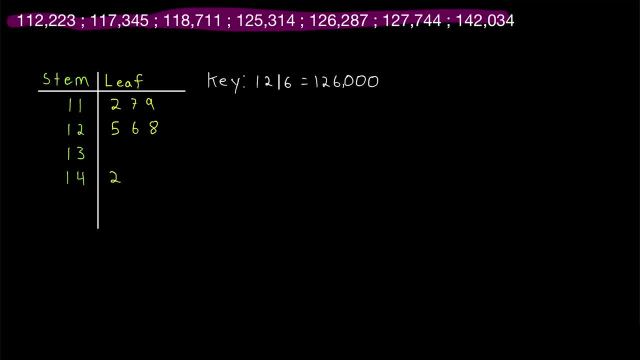 Then every data point in this set would have its own stem and they'd all have one leaf a piece. That would be a useless display. Instead, we use the stems to represent everything to the left of the thousands place. Doing that gives us a good handful of stems, But 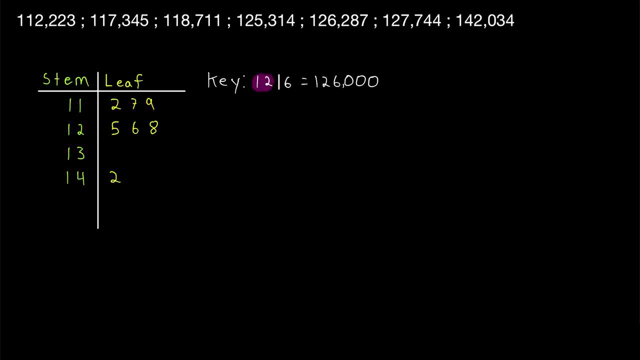 that means, of course, since we use the stems to represent everything to the left of the thousands place, The leaves have to represent the thousands place, which means I had to round all of these data points to the nearest thousand. So, for example, 125,000 314 was rounded to 125,000,. 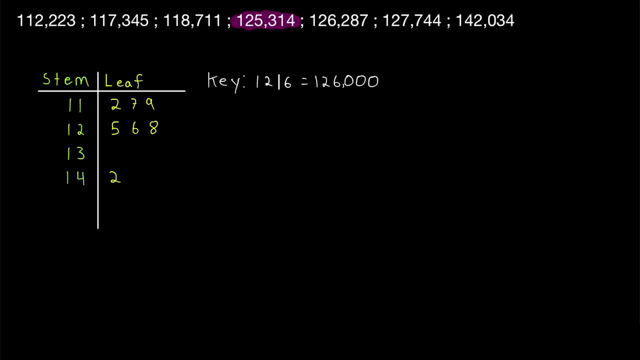 which we can see in the stem and leaf plot, in the 120,000 stem. And there it is with the five leaf, So that's 125,000.. Of course, when we do this sort of rounding, our stem and leaf plot no longer completely preserves the original data, but it does still.